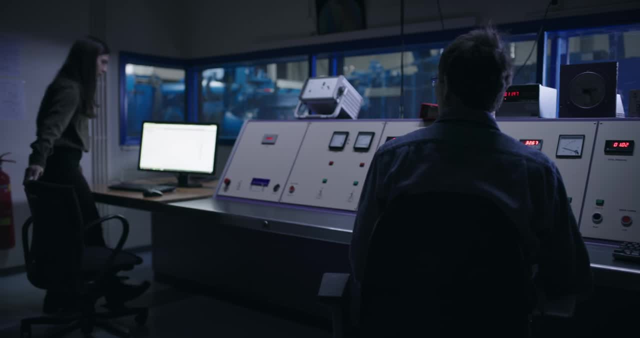 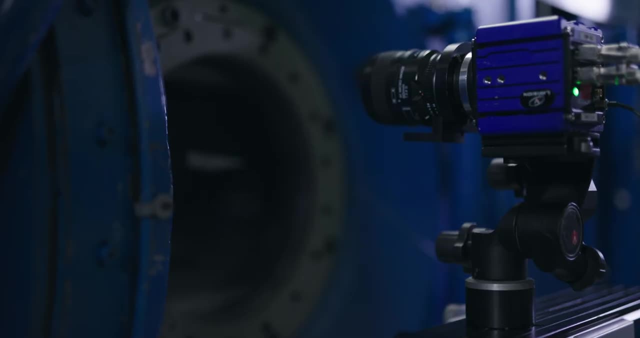 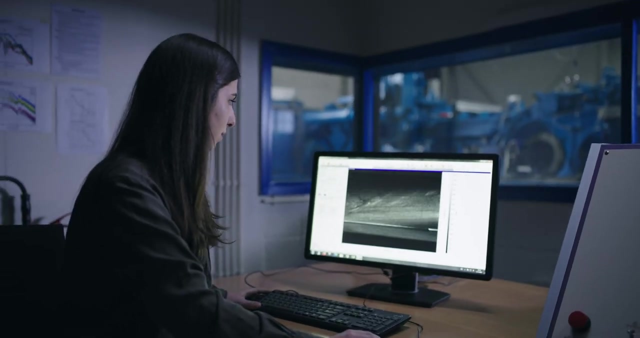 and supersonic air flows. We are using some advanced measurement techniques, such as PIV, as you can see in the wind tunnel set. My research is focused on shockwave boundary layer interactions and I aim to increase the efficiency of aircraft engines and turbine cascades. 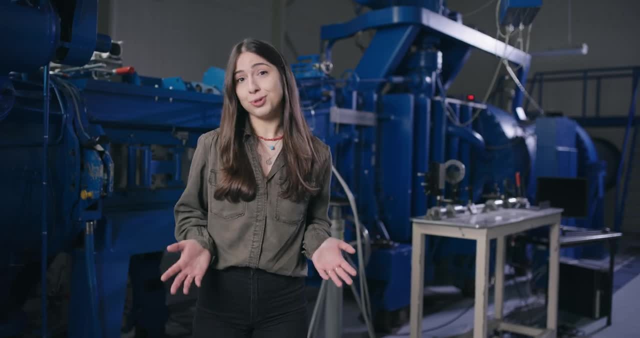 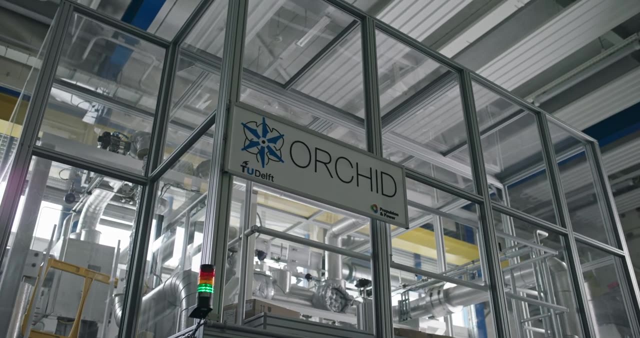 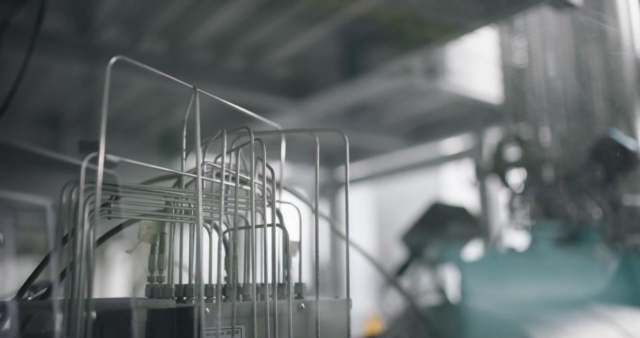 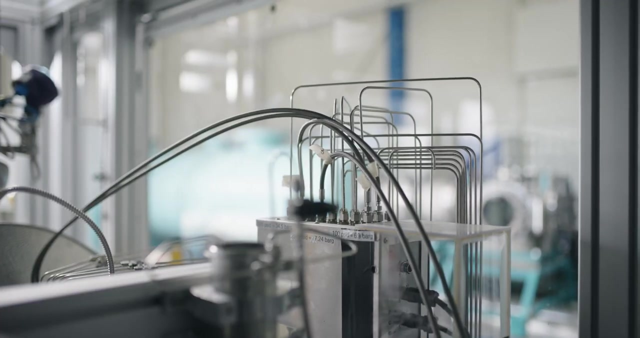 And with this research, we would like to contribute to sustainable aviation. This is ORCID, which stands for Organic Rankine Cycle Hybrid Integrated Device, a hybrid supersonic wind tunnel and turbo machinery test bench. This is where researchers investigate the use of waste heat to produce electricity, Heat that is generated by the engines of the. 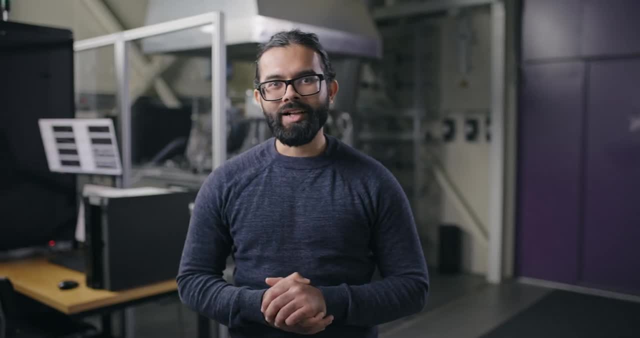 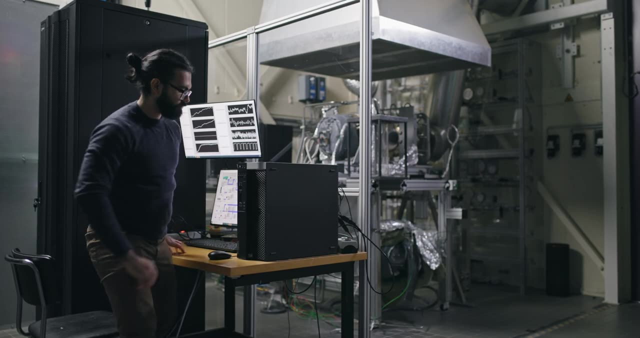 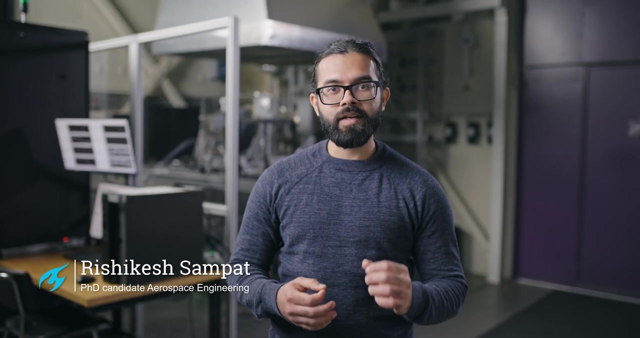 future is developed by researchers like Rishikesh. Welcome to the Clean Combustion Lab Over here. we are developing combustion technologies for low NOx and CO emissions. We not only work with conventional fuels, but also sustainable fuels such as hydrogen, and develop combustion devices for low emissions. 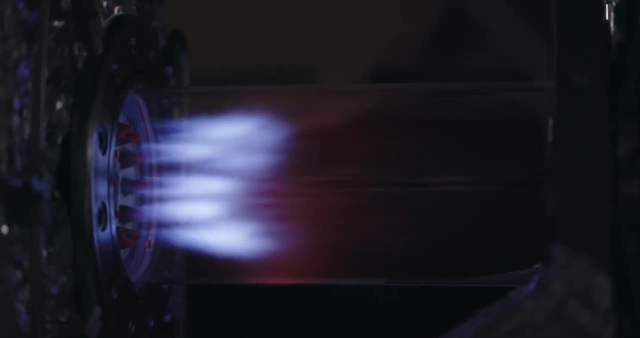 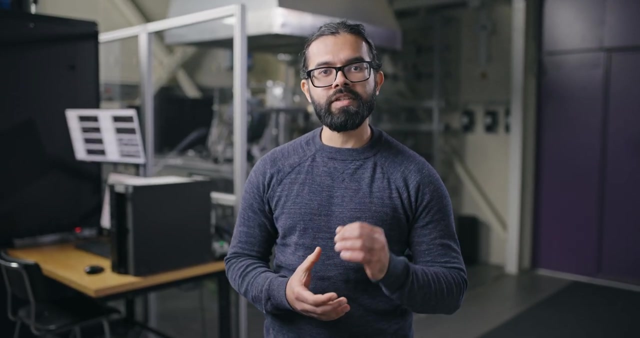 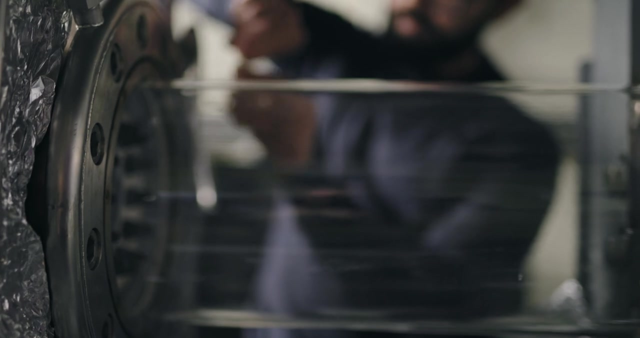 What you see running over here is the flameless combustor. Flameless combustion is a regime in which the reactions occur in a distributed manner. This regime also enables us to operate with extremely lean fuel air ratios. Typically, our measurements are done with optical diagnostic methods, which is why you see that the chamber 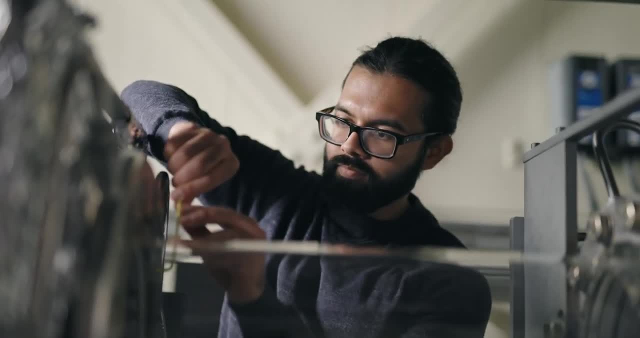 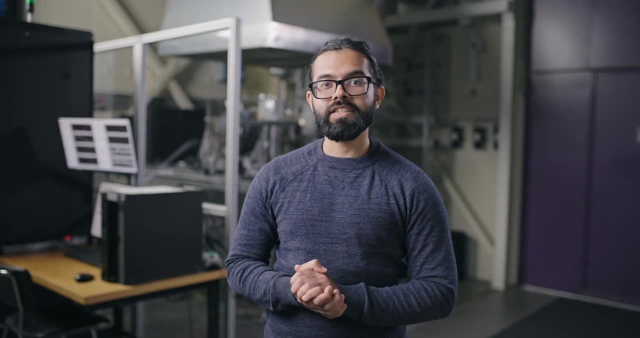 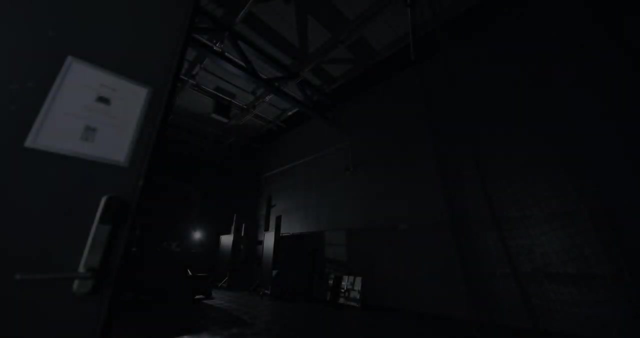 was designed to be fully transparent and is made of quartz. With the energy transition around the corner, I'm really looking forward to my contribution to sustainable aircraft by the development of clean combustion technologies. I'm Rishikesh and I'm here to talk to you about the Clean Combustion Lab. 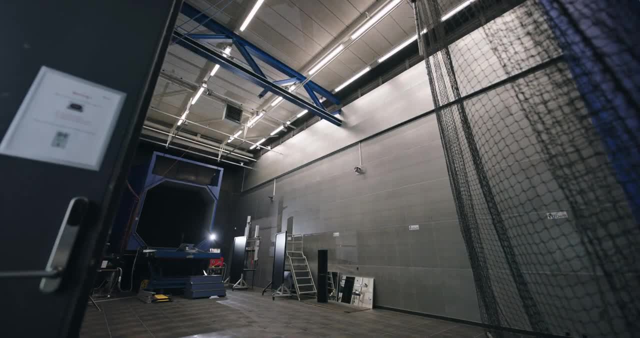 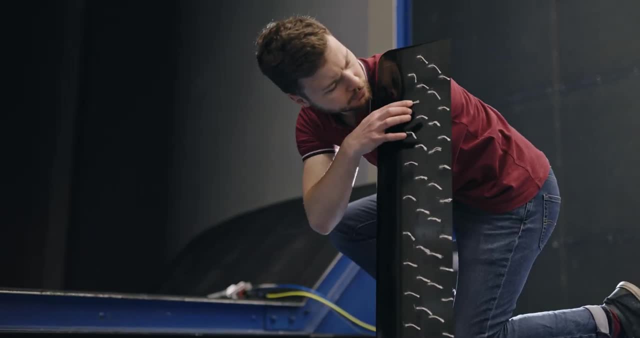 Our largest wind tunnel is the Open Jet Facility. It's used to test air flows around large scale objects like wind energy systems and UAVs, but also to improve sports aerodynamics for speed skaters, cyclists and even snowboarders, using particle image velocimetry. 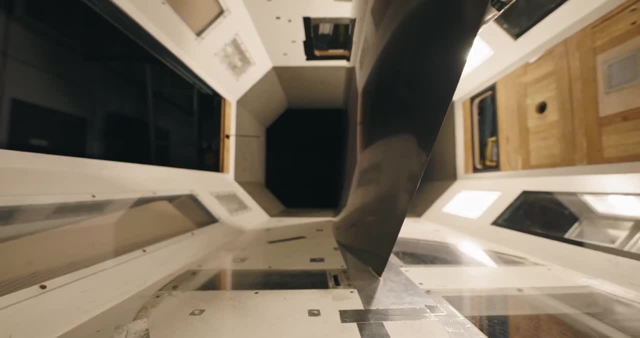 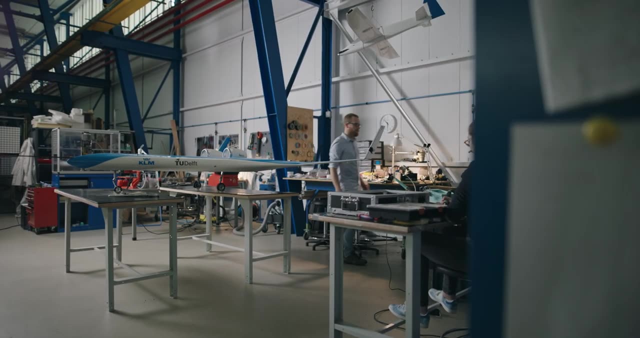 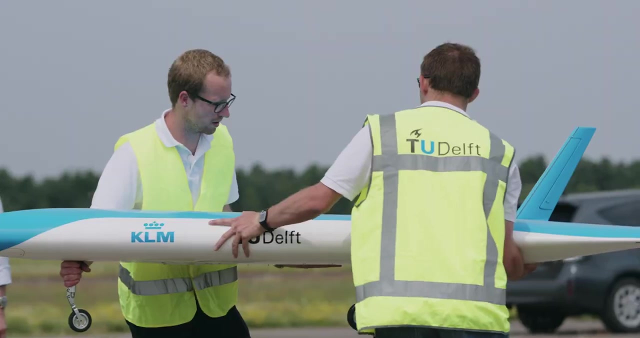 After testing components in the wind tunnel, the next step is to test an entire aircraft in the real world. The Scaled Flight Testing Lab is where we build and test scale models of new aircraft. designs such as the Flying V Scale models are essential to test what their flight characteristics are and whether they